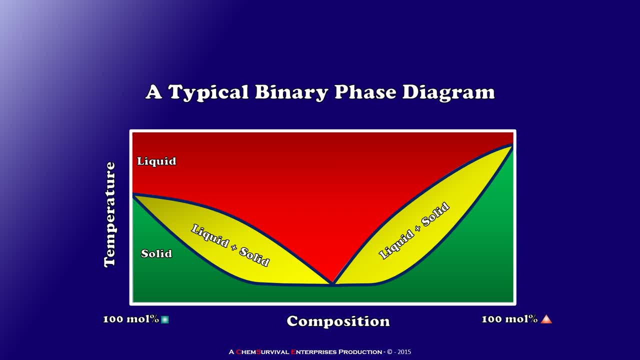 some interesting fields that we don't normally see in the phase diagrams of pure substances, specifically those yellow colored fields where we have liquid and solid coexisting over a range of temperatures. Now, if you google on the web for a binary phase diagram, you'll find that there are a number of different. 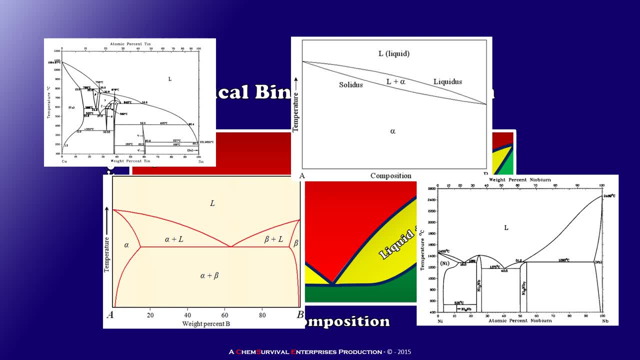 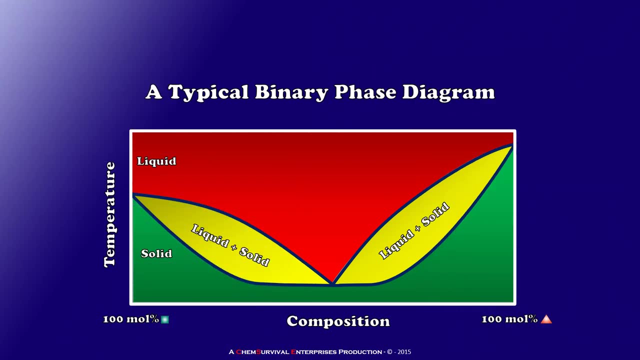 types of phase diagrams that you can use. You'll find a broad range of phase diagrams for a broad range of systems, some of which are very simple and others of which are incredibly complicated. So, for our purposes, we're going to stick to this very simple, idealized phase diagram that I've created for you here. So now, 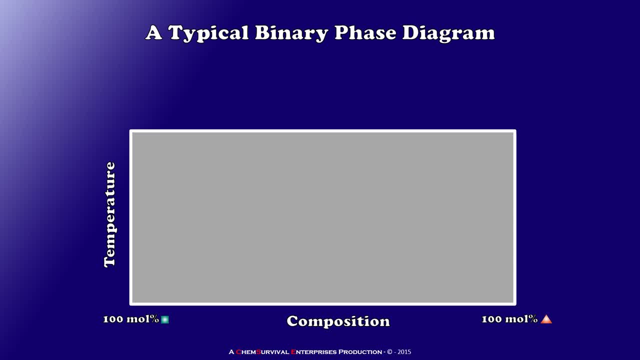 that we've had a look at this binary phase diagram, let's consider how it is built. To construct our binary phase diagram, we'll start with a pure material. Let's begin with our green square compound here. If I'm interested in the melting point of that pure compound, I can find it at the extreme left-hand side of my 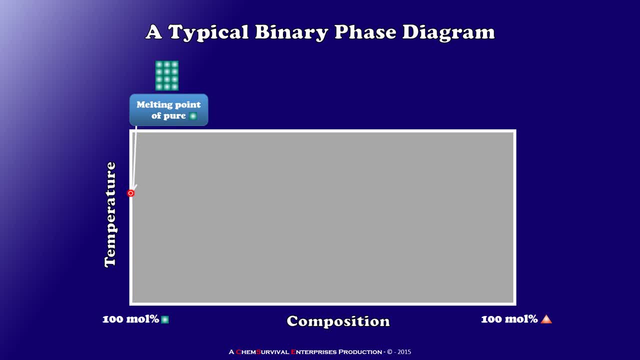 phase diagram. Because it's pure, we expect there to be only one single temperature at which solid and liquid can coexist. So as I heat a sample of this compound, I simply heat solid until I reach the melting temperature, and then I heat solid until I reach the melting temperature. 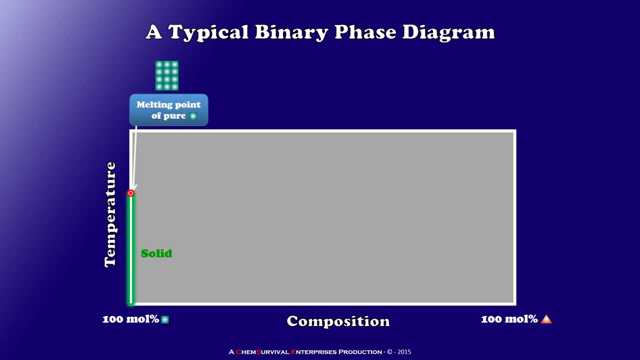 The melting transition then takes place at that temperature, and once it is complete, then I begin heating my liquid. But if I begin to mix in a small amount of a second compound- for example my compound, which is depicted by red triangles here- I see two important changes in the phase boundary. The first 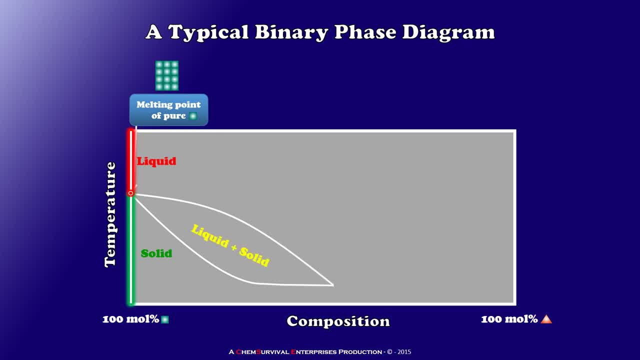 is that it goes downward. The melting point goes down when I add small amounts of my new compound to the mixture. And the second interesting characteristic is that it does not melt at a single temperature anymore, but rather over a range of temperatures, So I can take a. 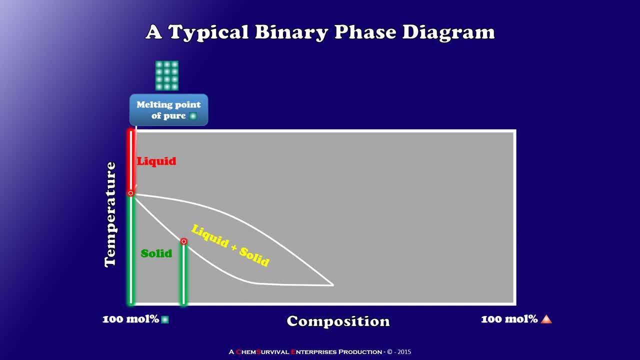 mixture of my red and green, let's say at this composition and heat the solid until the liquid begins to form. But as that melting process takes place, the temperature still changes, It goes up. So there's a range of temperatures over which this mixture of compounds can melt. 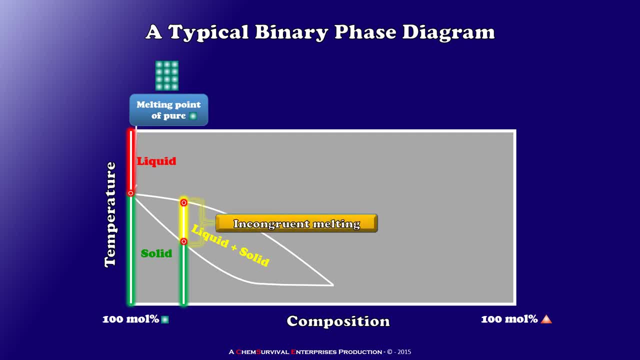 And we call this process incongruent melting. And it's caused by the fact that, as my mixture melts, one compound preferentially enters a liquid phase faster than the other. So the composition of the melting solid is continually changing as the process is taking place, thereby manifesting itself as a melting. 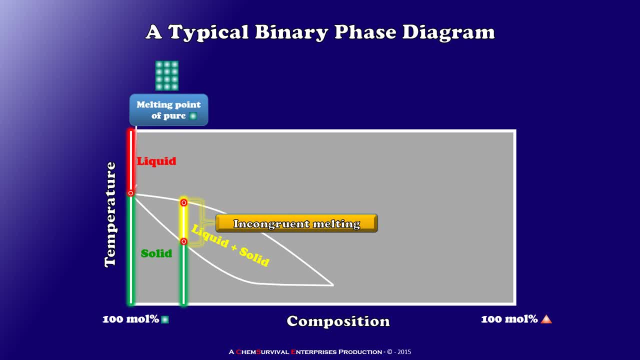 range rather than a melting point. And of course, if I continue heating, once melting is complete I simply heat the liquid again. So at this point we can think of this part of the diagram as my red compound acting as an impurity in my green compound. But eventually I reach a confluence somewhere near the middle. 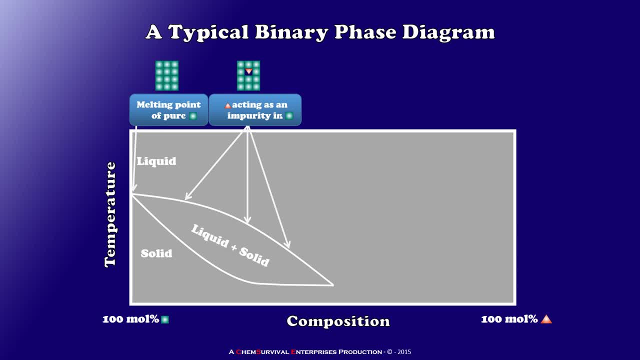 of the diagram, though not necessarily directly in the middle, as I've depicted it here. When this happens, we've reached what's known as the eutectic point. You'll notice that the eutectic point is the only point so far, besides pure green compound, at which 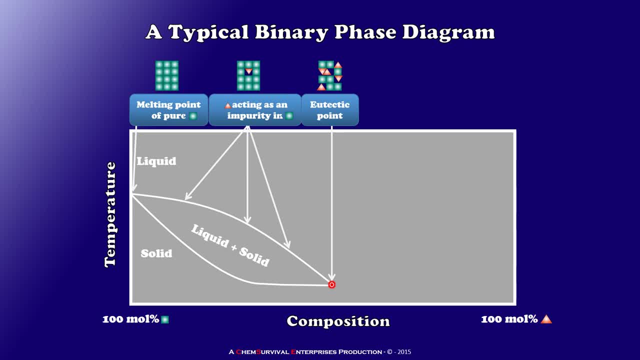 we have a single melting transition And it's also the lowest melting transition temperature possible, And this is the origin of the name eutectic. It's taken from Greek terms meaning easy and melting, So the eutectic mixture of these two is expected to melt. 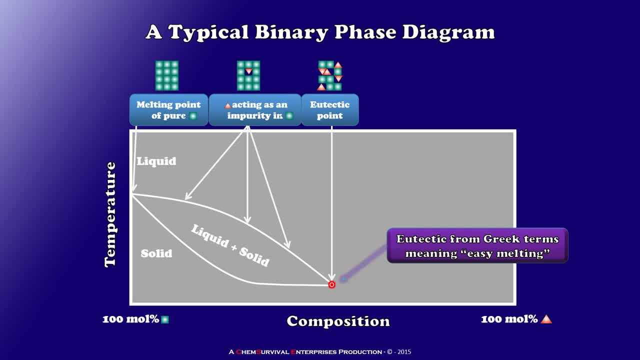 at a single temperature and also at the lowest temperature for any mixture of the two compounds. As I continue to add more and more red compound to my mixture, you'll see my melting point be the same. The melting point begins to increase again, eventually reaching the melting point of the 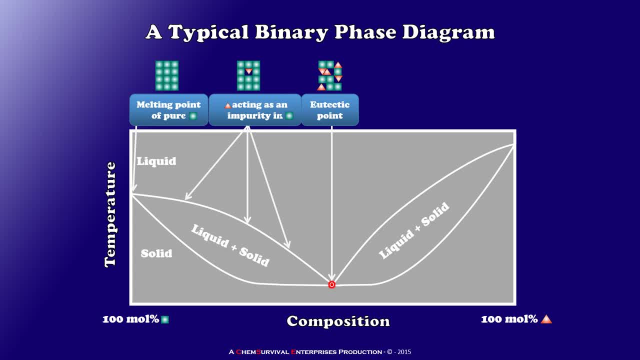 pure red compound. So I've created another region of my diagram where liquid and solid can coexist, but this time because of the green compound acting as an impurity in the red as opposed to vice versa, And, of course, as my concentration goes closer and closer to 100% red, I ultimately approach. 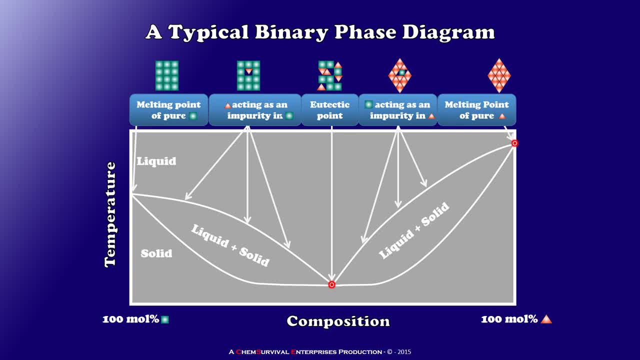 its melting point and we finally reach it at 100% red compound. So this is how we can think of binaries. This is how we can think of binary phase diagrams as simply being the contamination of one compound with another until we reach a eutectic, and then turning the tables on.